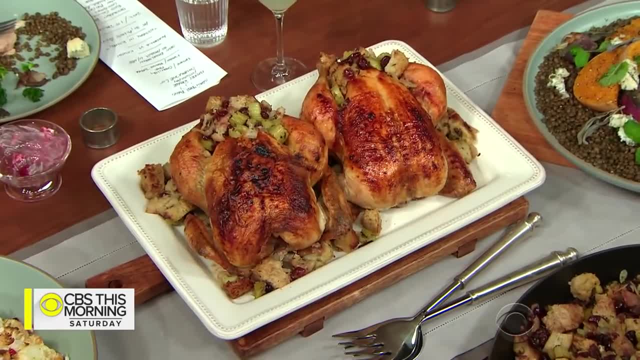 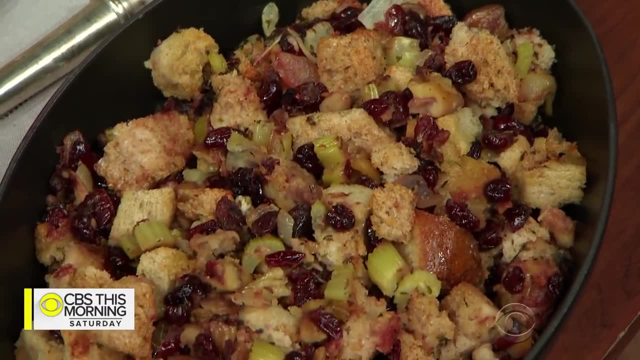 Okay, so the main thing is the roast chicken, Two big roast chicken and it's got a really wonderful stuffing made with sourdough, bread, caraway, Moist, moist, moist. Yeah, it is all about that. And then the sides are. I've got roasted butternut squash with. 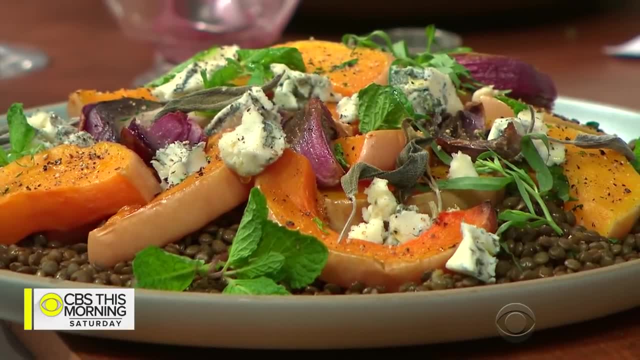 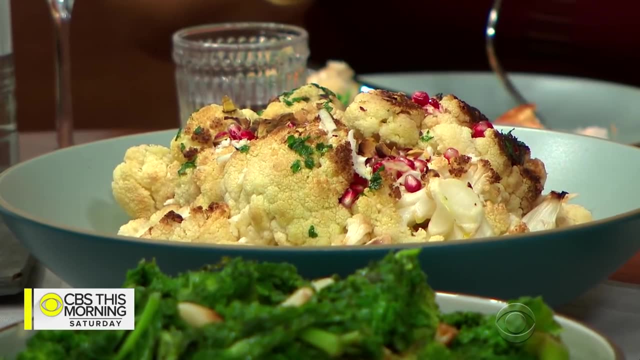 lentils, dolce latte and tons of herbs. There is broccoli and kale with fried garlic and cumin, roasted cauliflower and raw cauliflower, salad with pomegranates and pistachios, And this delightful little Oh, and that's a coriander, or cilantro, as you say here. 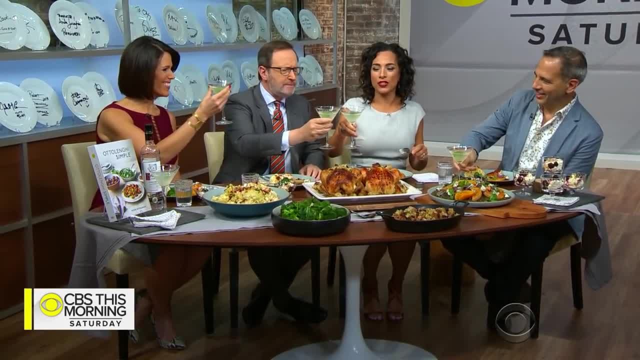 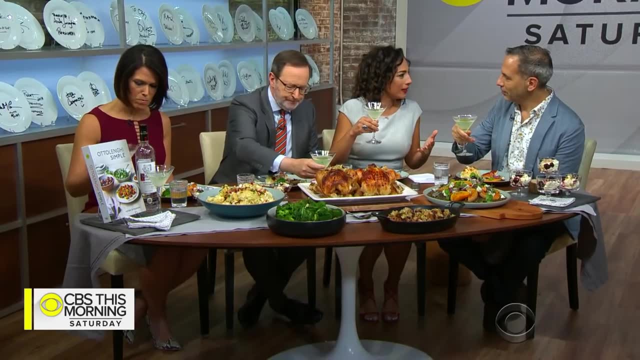 We say both. Okay, here we go. We say cheers, It is. We say cheers. So you say you had a self-professed. you say yourself that you were a happy kid. I was. So what made that so, and did the kitchen have anything to do with it? 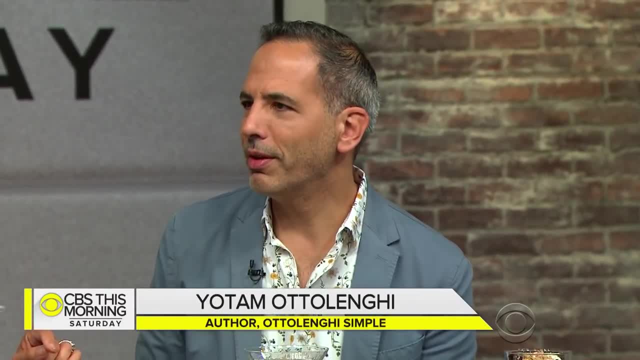 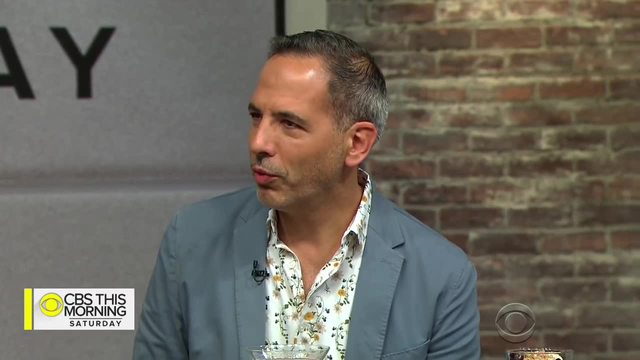 Well, to be honest, I mean, I've just. I grew up in Jerusalem, so I mean the food, as you know, in that part of the world is just Phenomenal To die for. You know lots of vegetables everywhere and you know Arabic food, as you know: the hummus. 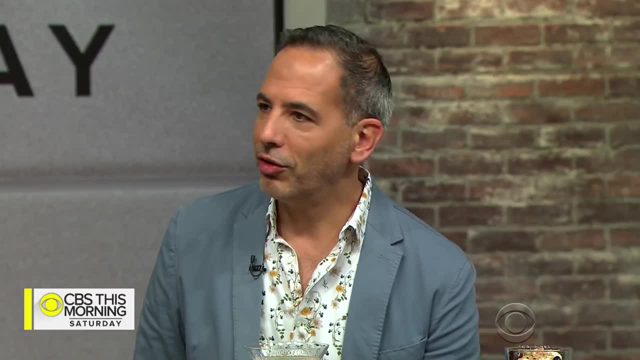 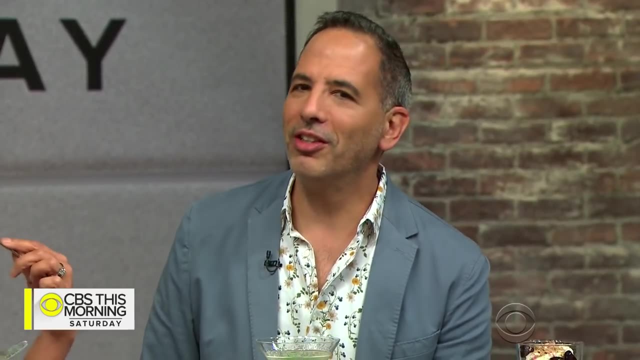 and the falafel and all the rest, And so I was really lucky to have been exposed to all these flavors. from childhood, I loved eating. Who doesn't? I still do. When I went to university, I realized that actually, if I won't cook for myself, nobody. 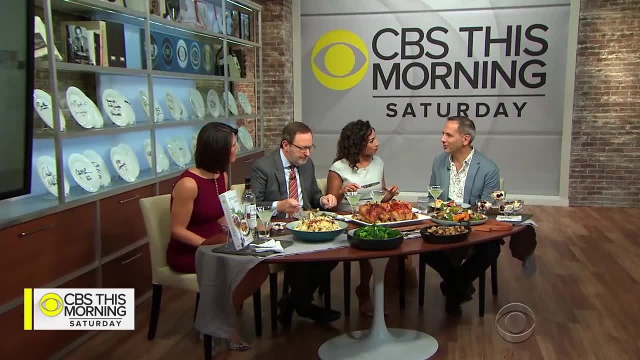 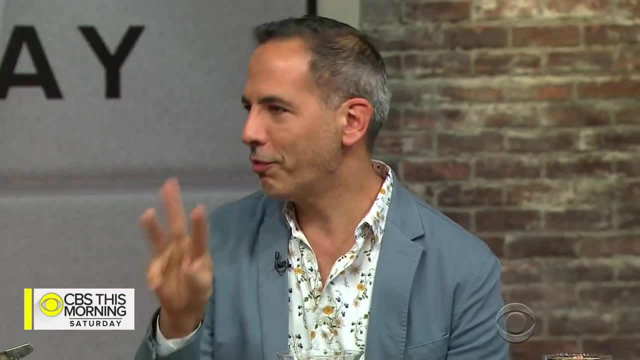 will cook for me. you know, I think that's the realization that every student has when they leave home. So I just started cooking and having people over, entertaining And the nice thing about cooking. I love three elements of cooking: Shopping for ingredients, cooking and then serving, because you get all these incredible. 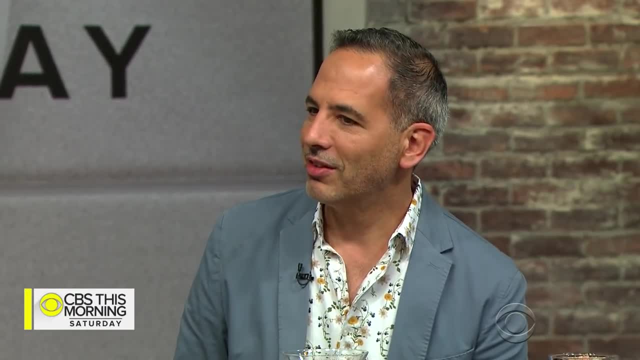 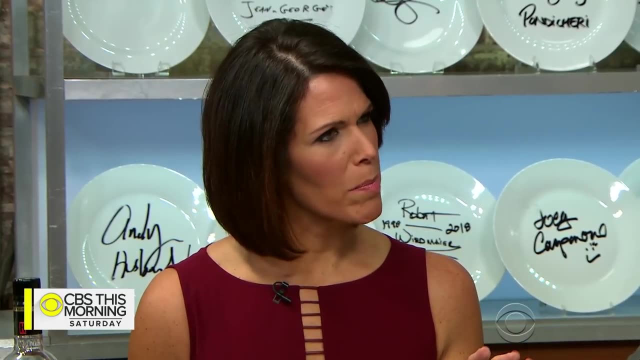 feedbacks. I mean, if you serve a good meal, Well, I could do without shopping, So that's how I fell in love with it. When you talk about studying at university, you had your master's degree in philosophy. Your parents come from this academic background. 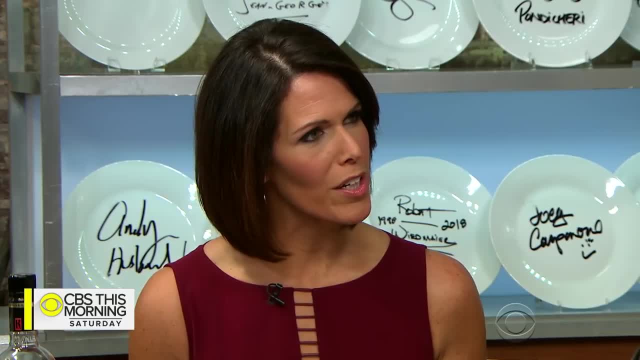 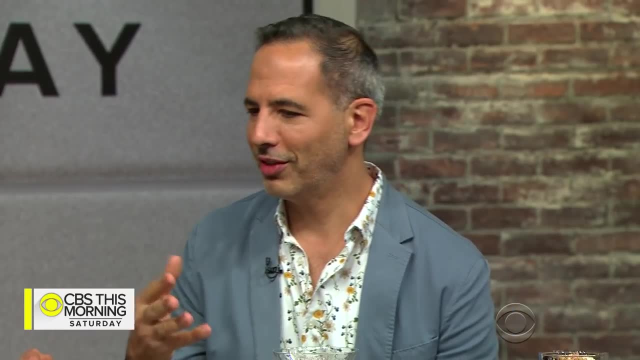 How did you tell them that you knew that you needed to go into the world of cooking? That was a bit painful, So I had my dissertation when I finished studying at university. I sent it through the post, as you did in the 90s. 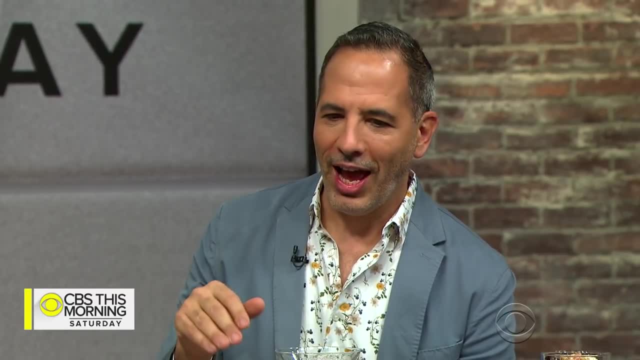 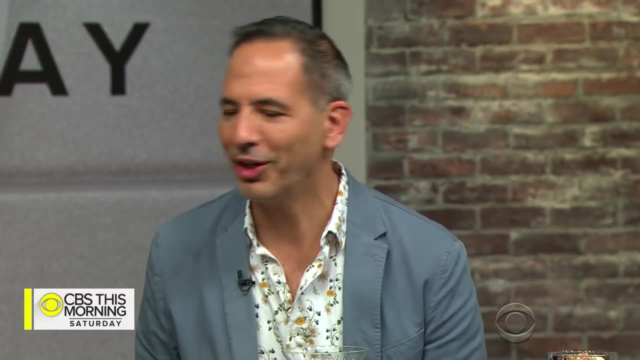 Do you remember? To my parents? To my parents? yeah, because I was living in Europe at the time And inside there was a little note. I went there, you go, there's my dissertation, I finished my degrees, But actually now I'm taking some time off and I'm going to learn how to cook. 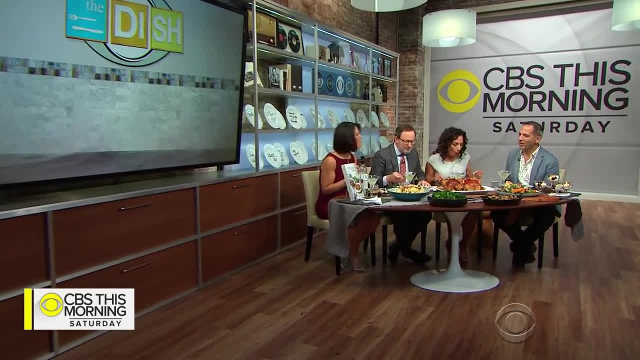 What did they say? That went over well. That didn't go down very well. So you know my dad is, you know he's the gentlest, nicest person. He said to me. I don't know if that's advisable. 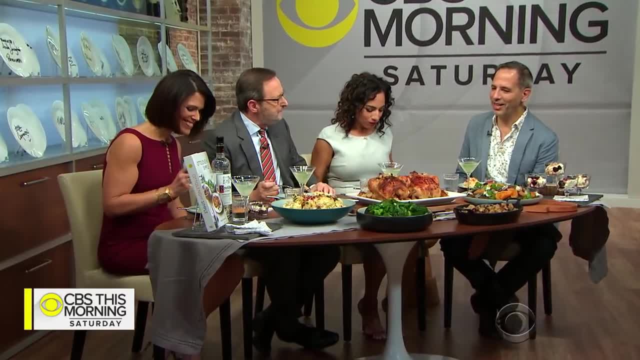 He's changed his mind since. right, He has changed his mind, yeah, I mean, you know he's had quite a few years to get used to the idea and he's seen what I've created and how much joy I'm getting. 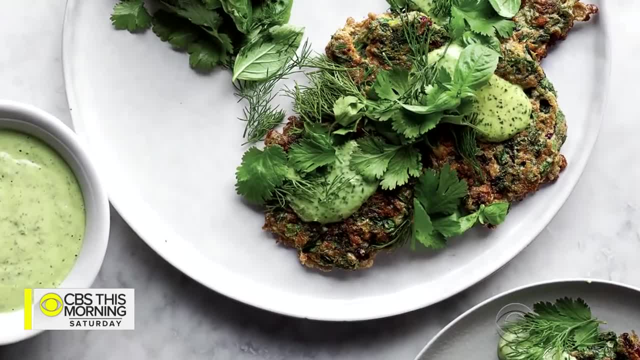 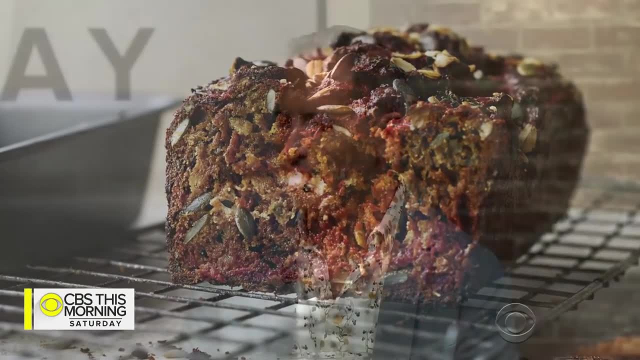 But in the beginning you described yourself as an oddball in the kitchen And you almost quit. Yeah, Kitchens are just hard. Yes, You know, it's like being it's very regimented. There's a lot of shouting and screaming going on. 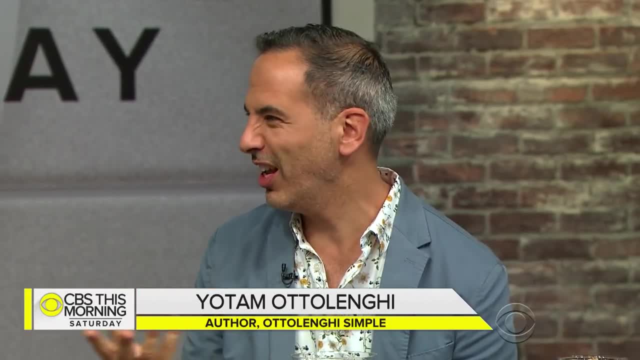 You need to get all the food out on time. So if you're you know slightly, don't fit in, it's difficult. So, yeah, I almost left, But then I discovered that I could choose my own place so I could look. I found places that I really enjoyed working at, And that's what I always tell young chefs these days: Don't work where you don't like to work. Work where you don't like to work. Work where you don't like to work. 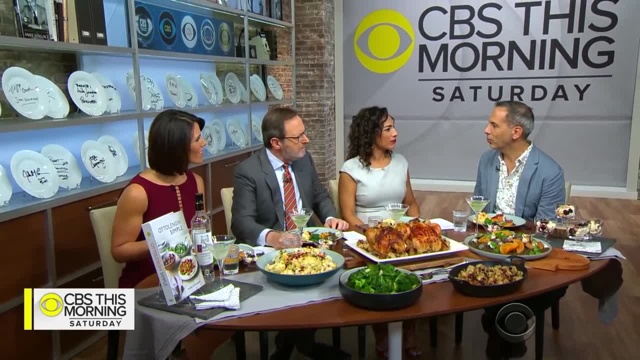 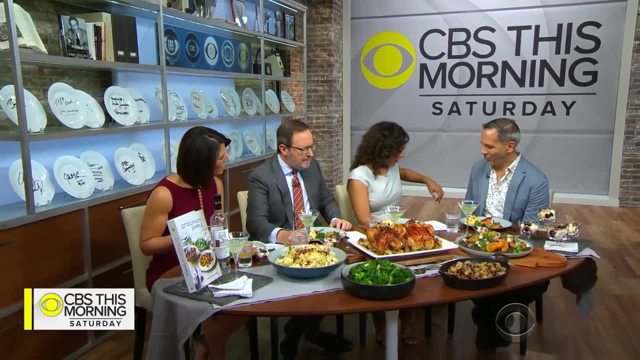 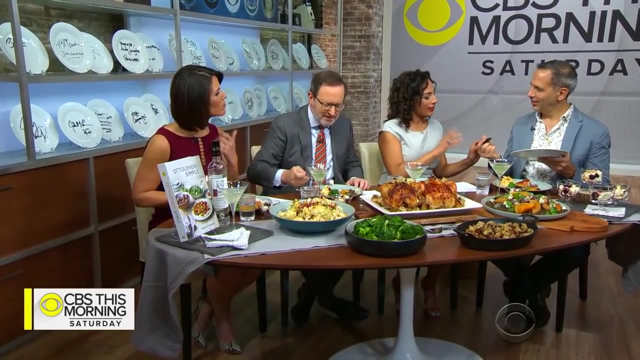 Work in good restaurants where you're being respected and you enjoy going to work in the morning, Otherwise kind of what's the point? And you have to respect yourself. I love that. I love everything about you, Tom. But as we finish up our meal and our drink, I would love for you to sign the dish and 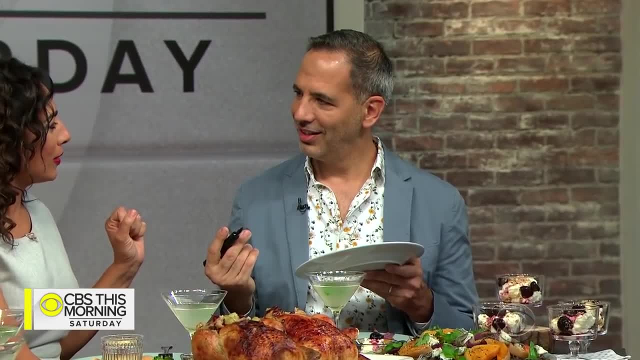 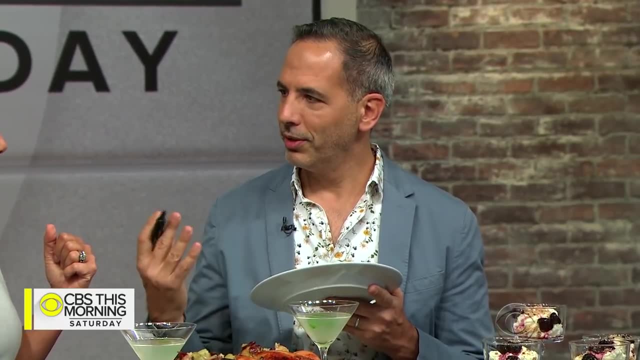 think about. if there's any one person that you would love to share this meal with, Who would it be? So there's an Argentinian chef called Francis Melman. He lives- yeah, he's- from Patagonia. He's from Patagonia down south. 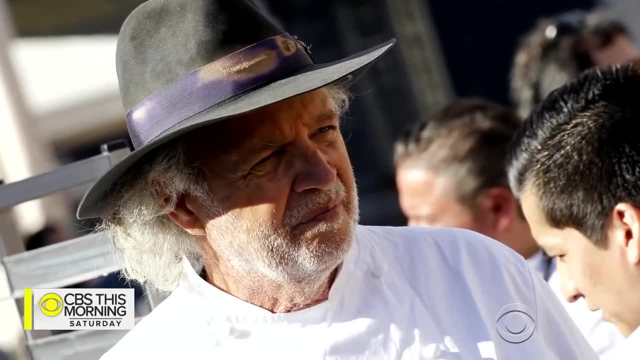 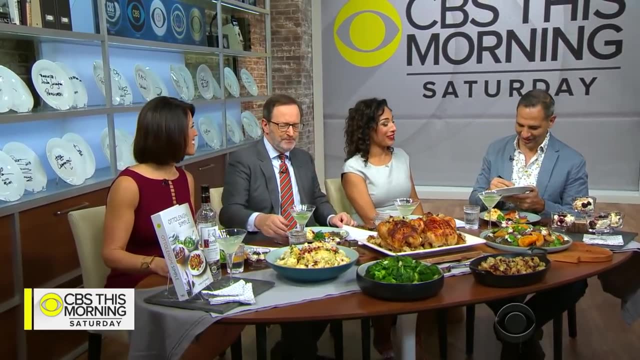 And he does incredible things on a barbecue and grill. I've only seen him once, met him once for like three minutes. That's the person I'd love to have. Wow, Great choice That is. I love it. Well, Chef Tom Otolengue, we appreciate you coming with us. 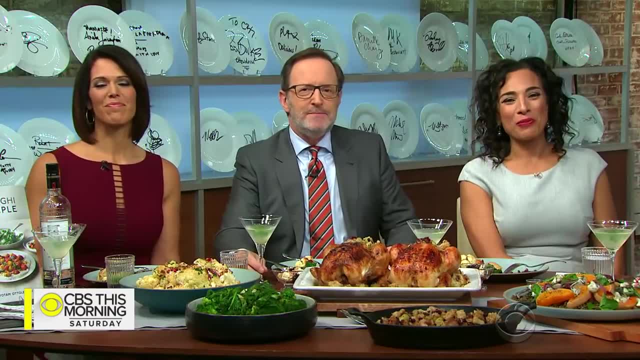 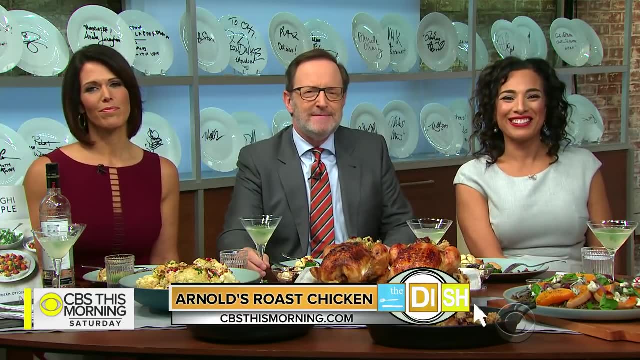 Thank you so much To share a meal. This was great, Awesome. And for more on the chef and his fabulous dish- ours as well- head to our website at cbsthismorningcom. 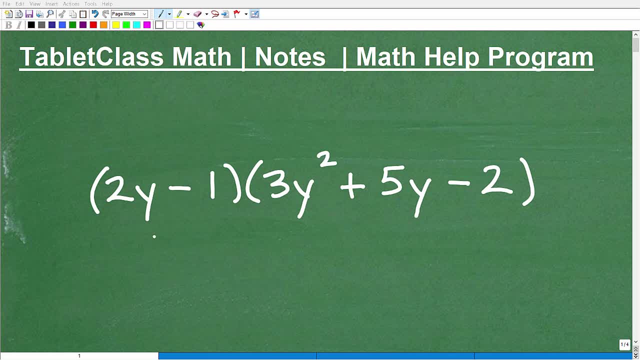 Okay, let's talk about how to multiply these polynomials here. So we have 2y minus 1 and we're going to multiply it by 3y squared plus 5y minus 2.. Okay, so we have a binomial being multiplied.